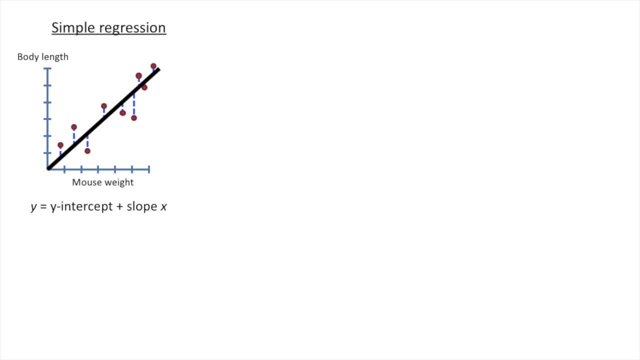 You might recall from the StatQuest on linear regression that simple regression is just fitting a line to data. We're interested in the R-squared and the p-value to evaluate how well that line fits the data. In that same StatQuest I also showed you how to fit a plane to data. 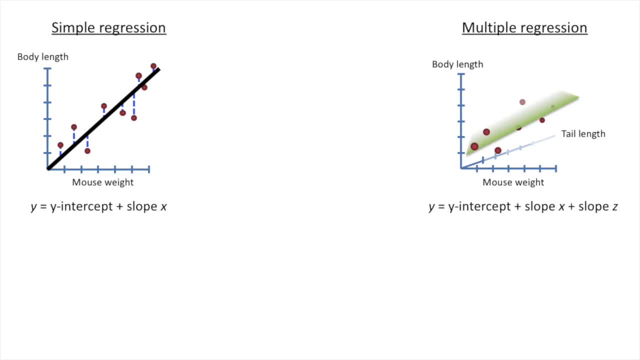 Well, that's what multiple regression is. You fit a plane or some higher dimensional object to your data. A term like higher dimensional object sounds really fancy and complicated, but it's not. All it means is that we're adding additional data to the model. 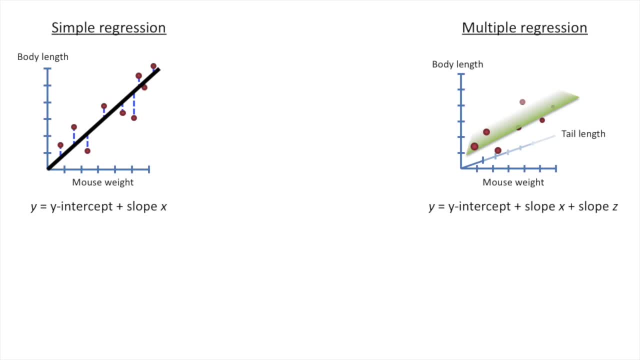 In the previous example. all that meant was that, instead of just modeling body length by mouse weight, we modeled body length using mouse weight and tail length, If we added additional factors like the amount of food eaten or the amount of time spent running on a wheel. 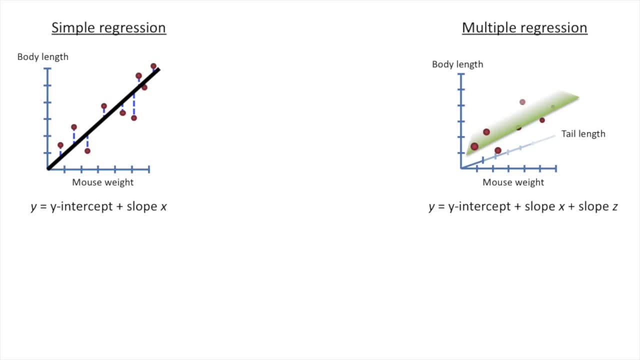 well, those would be considered additional dimensions, but they're really just additional pieces of data that we can add to our fancy equation. So from the StatQuest on linear regression, you may remember, the first thing we did was calculate R-squared. 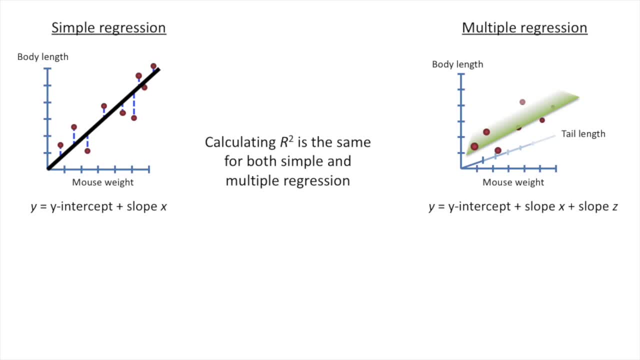 Well, the good news is that calculating R-squared is the exact same for both simple regression and multiple regression. There's absolutely no difference. Here's the equation for R-squared and we plug in the values for the sums of squares around the fit. 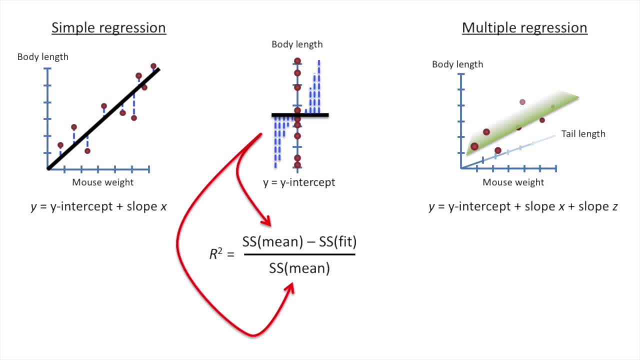 and then we plug in the sums of squares around the mean value for the body length, Regardless of how much data we have, additional data we add to our fancy equation. if we're using it to predict body length, then we use the sums of squares around the body length. One caveat is for multiple regression: you adjust. 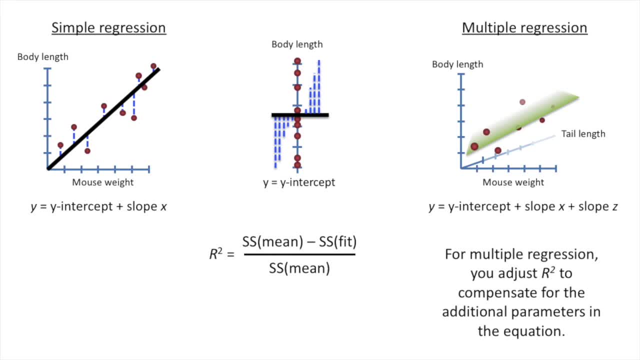 r-squared to compensate for the additional parameters in the equation. We covered this in the stat quest for linear regression, so it's no big deal. Now we want to calculate a p-value for our r-squared. Calculating f and the p-value is pretty much the same. You plug in the sums of. 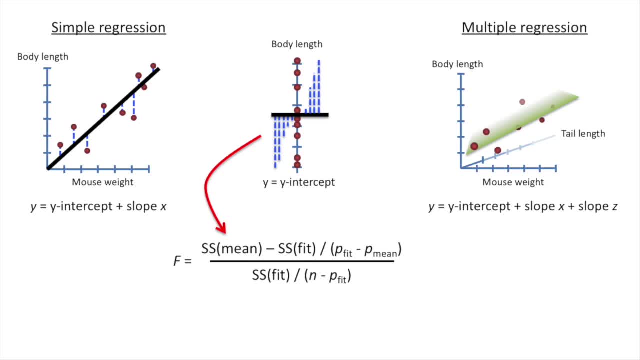 squares around the fit and then you plug in the sums of squares around the mean. For simple regression, p-fit equals 2, because we have two parameters in the equation that least squares has to estimate And for this specific example, the multiple regression version of p-fit equals 3,.